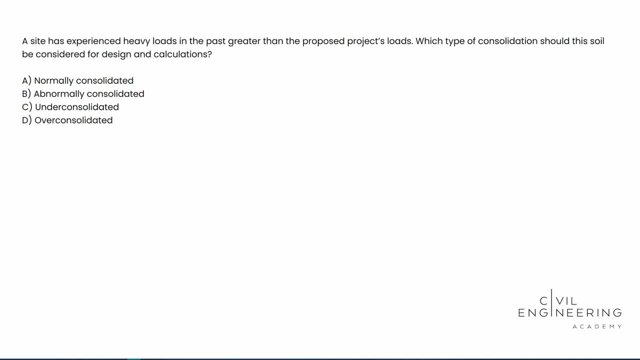 under-consolidated and over-consolidated. So if we're looking for some reading material, we need to look in the PE Reference Handbook And at the time of this recording, version 1.2 is the latest and greatest. We're going to be looking in chapter 3, so geotechnical is going. 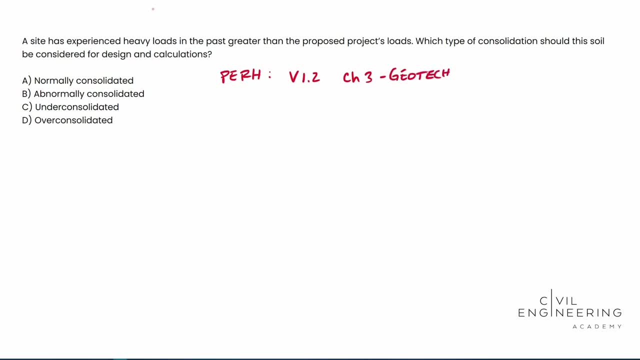 to be the section that we need to look, And whenever we go there there's actually no real answer, It's just general information that may happen. So we're going to be looking at the PE Reference Handbook. It's going to help us kind of hint around the answer, But there's really two different. 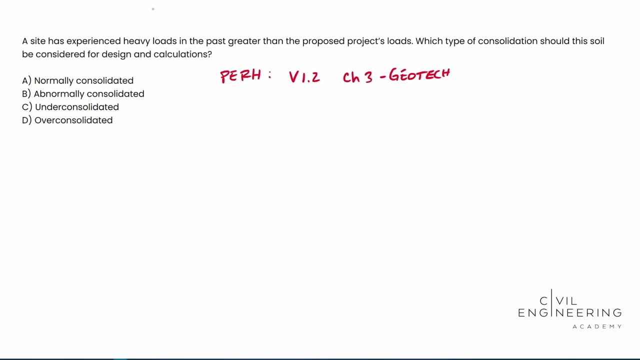 types of consolidation. There's normally consolidated and over-consolidated, So kind of, keep that in the back of your mind. There's only two, so you can go ahead and eliminate B and C. it looks like We can go ahead and knock those out And then you get a 50-50 shot. But let's. 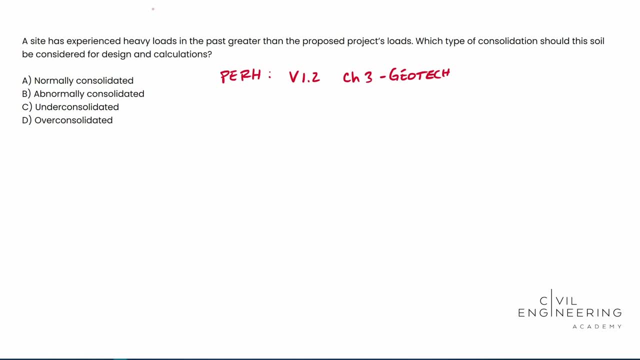 go ahead and solve this one. So think about it. Normally consolidated is virgin clay that has never experienced vertical stress higher than its current position or condition. So think about this. Let's say you're putting a tire center over what used to be farmland. Well, that farmland. 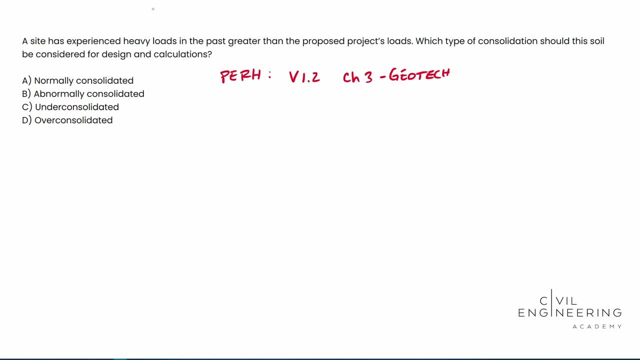 assuming that it didn't have heavy loads on it beforehand- it just had cows grazing or goats or what have you- then that would be the normally consolidated clay. But whenever you have something really heavy, that was on it and then you put something a little bit lighter, let's say you: 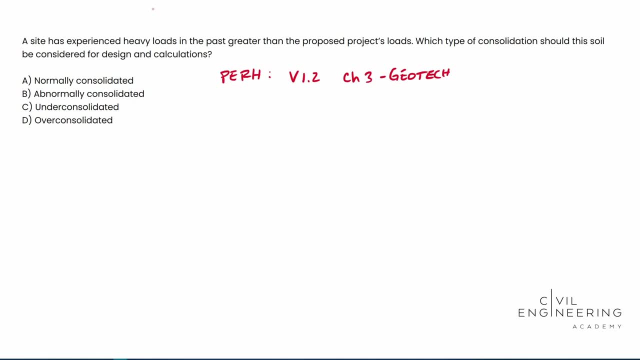 take that heavy object off and then you replace it with something lighter, like our proposed project loads. that's going to be over-consolidated clay. So the real definition of over-consolidated clay is a clay that has already experienced stress, that no longer exists, So like glaciers and things like that. So you're essentially 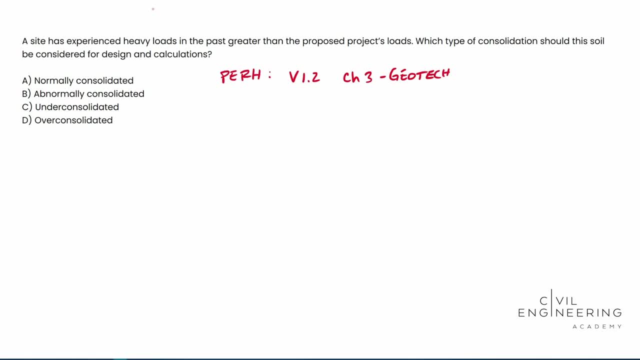 it once had this really heavy weight on top of it. You take it off, so it's already consolidated, It's already really jam-packed, And then you put your new project on top of it. So that's kind of what that means. So this one right here. we had heavy loads in the past, greater than the. proposed project's loads over-consolidated. So that's kind of what that means. So this one right here. we had heavy loads in the past greater than the proposed project's loads over-consolidated. So this one right here. we had heavy loads in the past greater than the proposed project's loads over-consolidated. 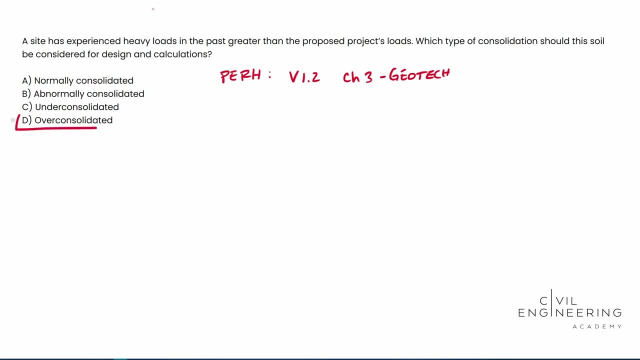 It's going to be our answer for this one, So hope it clears some things up. Hope that makes sense. The answer's going to be D and we'll catch you next time.